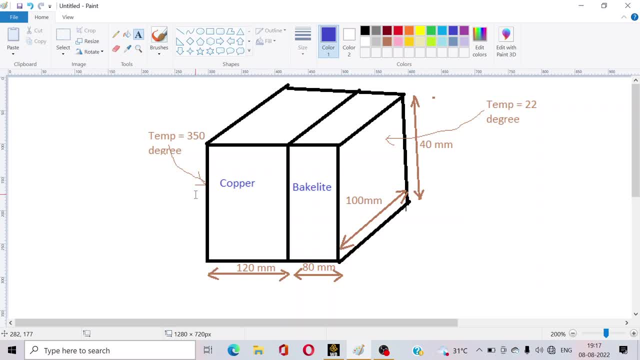 temperature of this surface is 22 degree, So the conduction will take place from this direction to this direction, Heat will be transferred from this direction to this direction right, And the temperature of different sections of the slab will be different and we will have to determine. 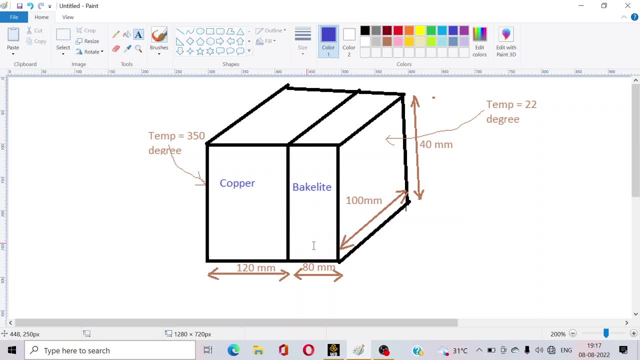 the temperature at the junction of these two slab. okay, And you can see the dimension: the cross section of the slab is 100 mm into 40 mm and the bakelite slab is 80 mm long and copper slab is 120 mm long. okay, Let's open the ANSYS workbench software. I have already opened it on my PC. 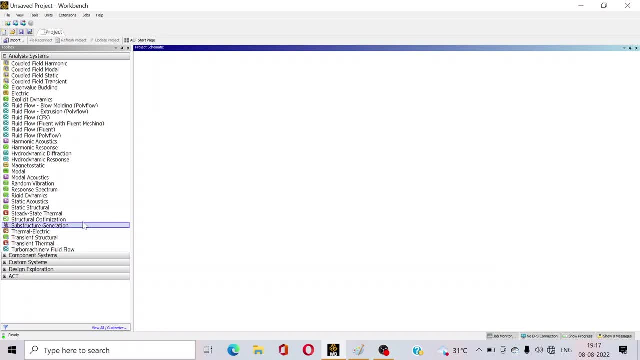 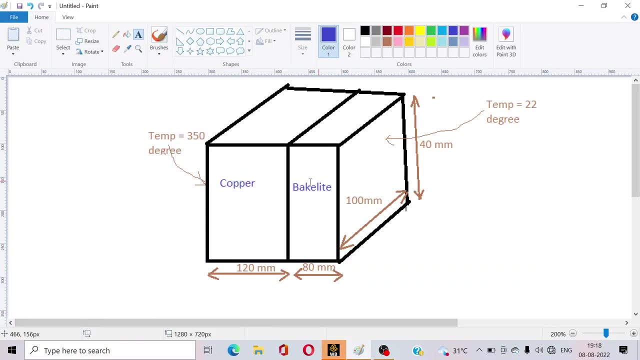 So here it is a time independent problem, so that we have to select the steady state thermal option right. Just double click on it. Okay, you can see that and you have already seen that the block is made up with the copper and bakelite right. So we know that at engineering. 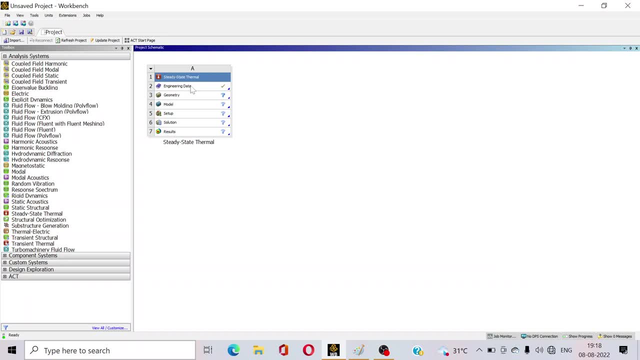 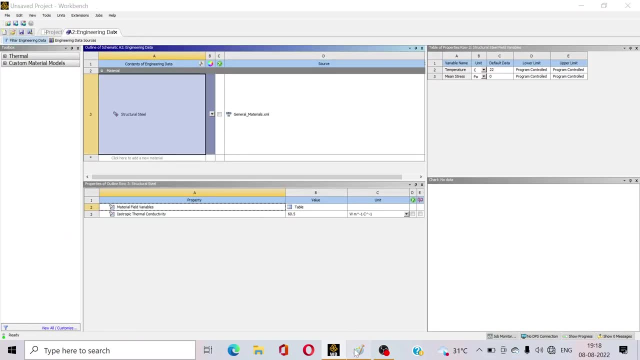 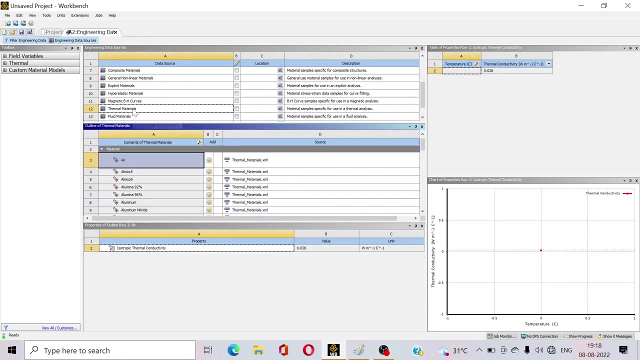 data section structural steel material. by default it was selected by the software right Here the materials are different. One material is copper and another material is bakelite. So just open engineering data section and go to the engineering data source and again go to the thermal material. 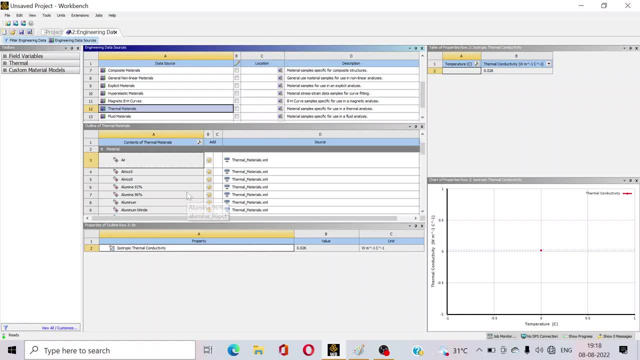 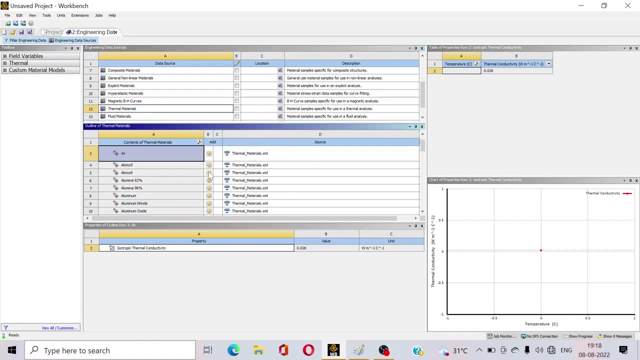 and this is nothing but where the new material, right. So here you can see the bakelite option. just click on this plus sign. it will be appeared. okay. And again we have to select the copper. This is copper. Click on this plus sign. Okay, the work is done here, right? 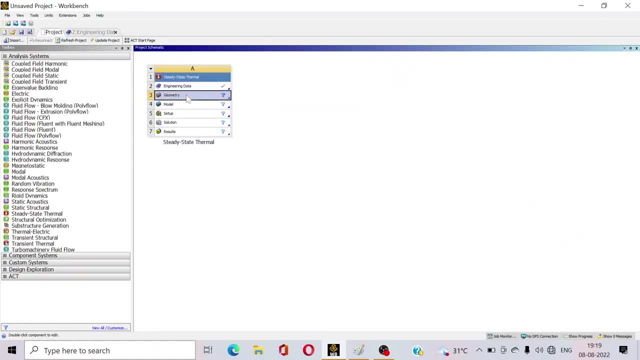 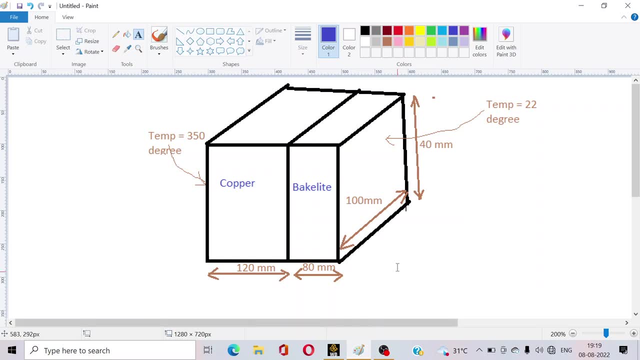 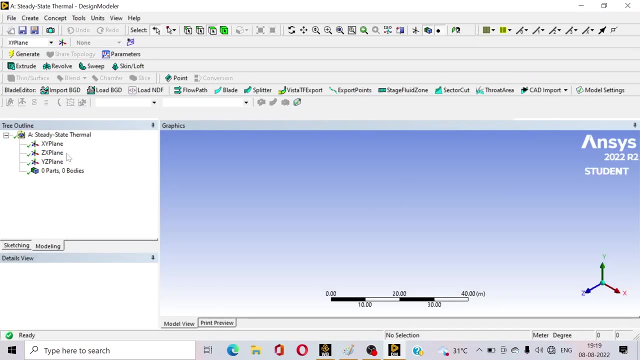 Then go to the project and just double click on geometry, because we have to draw this problem first, right? so in the geometry section we'll first draw the cross section, that is, 100 mm by 40 mm, right? so select any of this plane- i am selecting x, y plane- and just go to the unit and select. 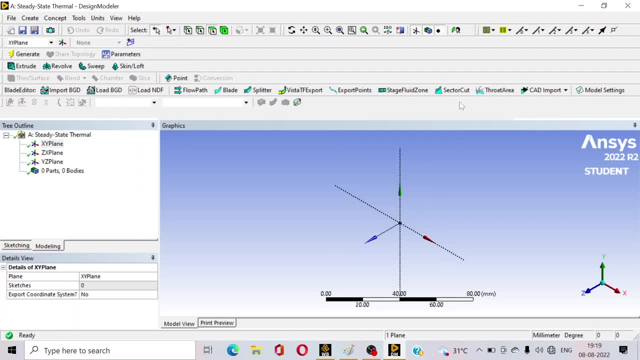 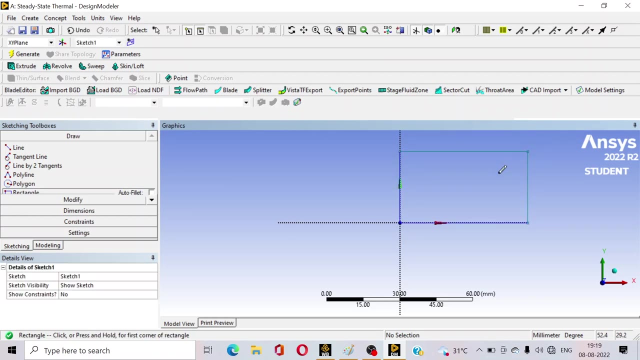 millimeter, right. so it is a 3d interface. let me convert it into the 2d. so just click this option. look at the face option. so this is your x- y plane. now go to the sketching, select rectangle and draw our rectangle. then go to the dimension, click this side of the dimension and click this. 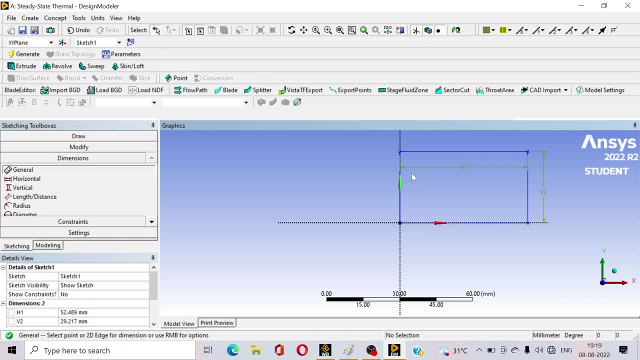 side of the dimension, you can see that two dimension is already created, two dimensions: one is h1 and another one is a v2. so we know that the cross section of our slab is 100 by 40. so type just type 100 here and just type 40 here and press enter. 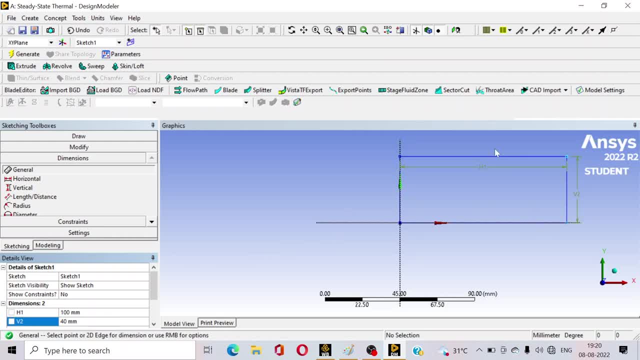 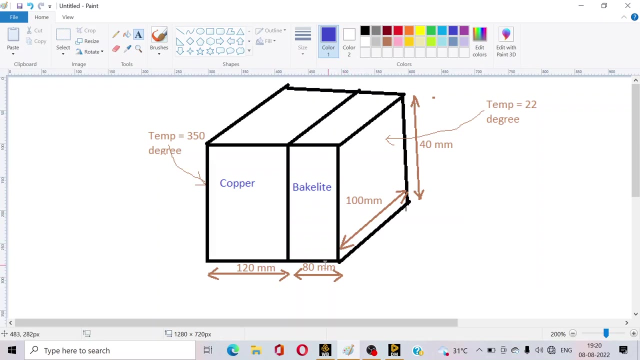 okay, so we have drawn our rectangle of two sides, 100 mm and 40 mm. okay, now go to the problem. you can see that we have made this cross section. now make an extrusion of 120 mm. this is for the copper one. okay, so go to the geometry again. 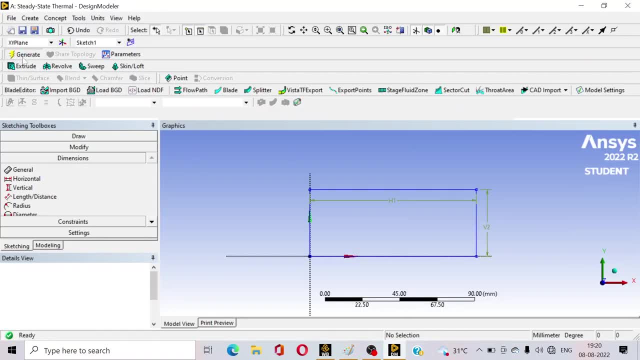 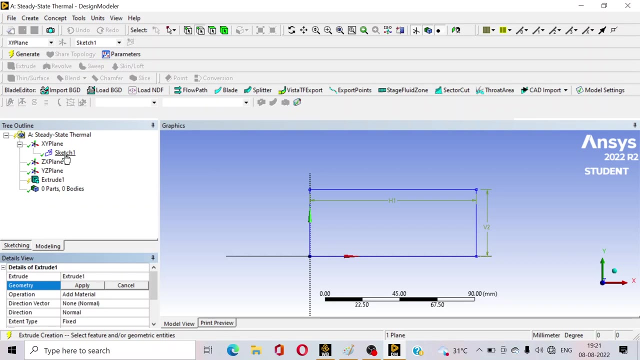 okay, we have drawn it. so just click on generate so that the sketch will be generated. okay, here you can see that under x, y, plane, sketch one is generated. okay, now go to the extrude option right now. click on sketch one and here click on apply, so case sketch one is applied for the extrusion, and what is the value of extrusion? 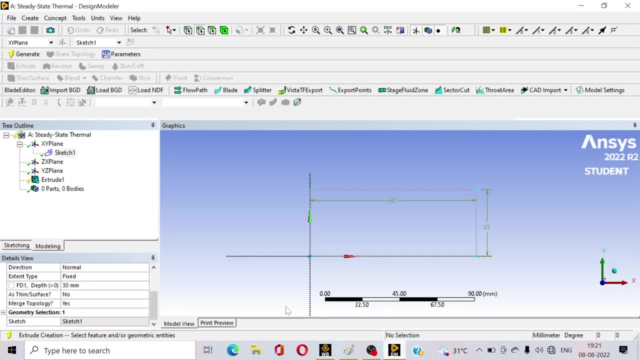 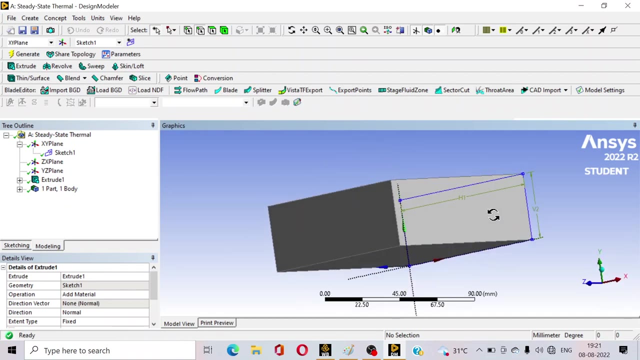 this is nothing but 120 mm. okay, so just click here 120 mm, just type 120. okay, then press enter and click generate. you can see that a solid is generated already. okay, this is nothing but your copper slab. okay, this is the copper slab now, from here, from. 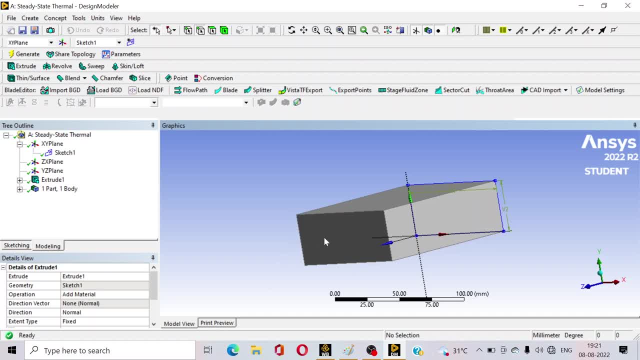 this surface. another slab is there and this is that is nothing but the bakelite slab. okay, so just click this surface. click this surface. okay, to select the surface, just click this option. okay, now click this surface. okay, and look at this surface. okay, so, as the cross section of 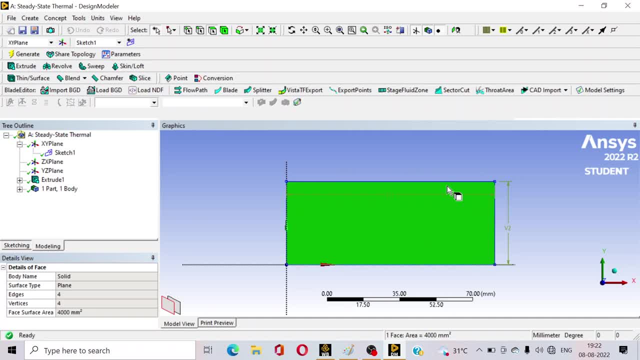 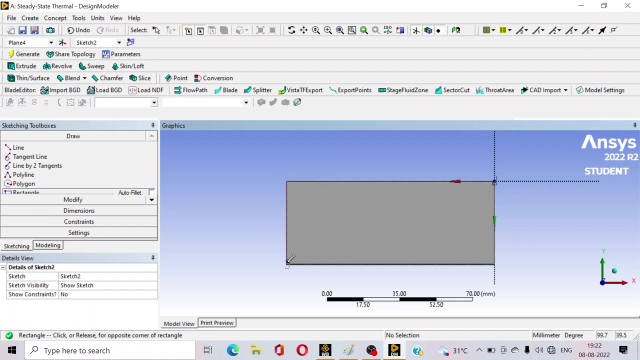 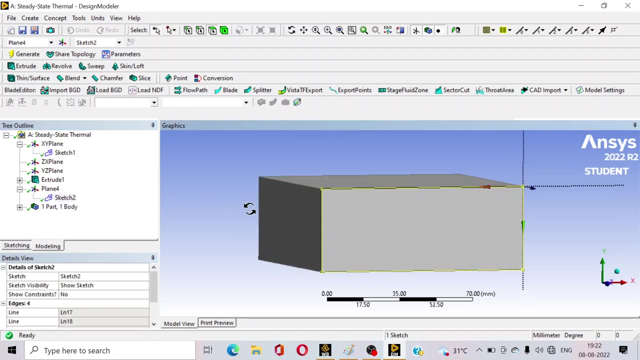 the bakelite slab is same as this cross section of the copper slab slab, so that we will make a rectangle again of same dimension. right, so make a rectangle of same dimension. okay, now click on generate. okay, you can see that automatically a different plane and sketch two is generated, and 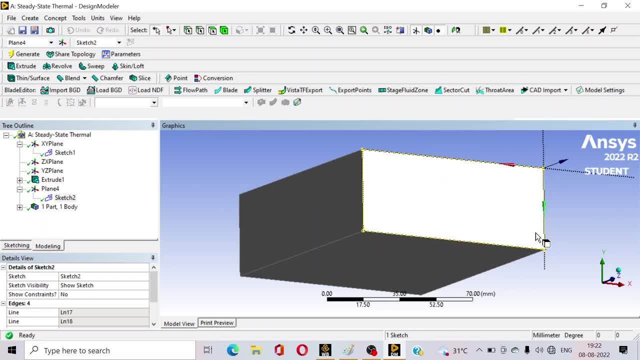 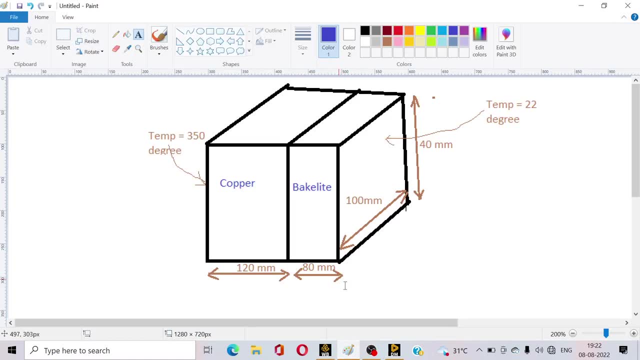 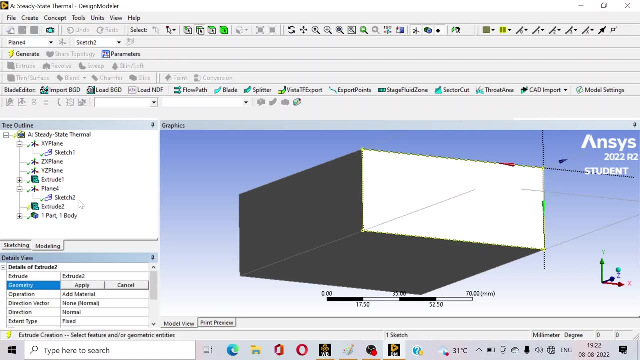 this is nothing but your the cross section of your bakelite slab. okay, now make it extrusion. okay, of 80 mm. right, extrude this sketch to 80 mm. now go to the extrude, select sketch two and then apply and this is type 80.. now see, here is a trick. you can see the option, the operations there are. 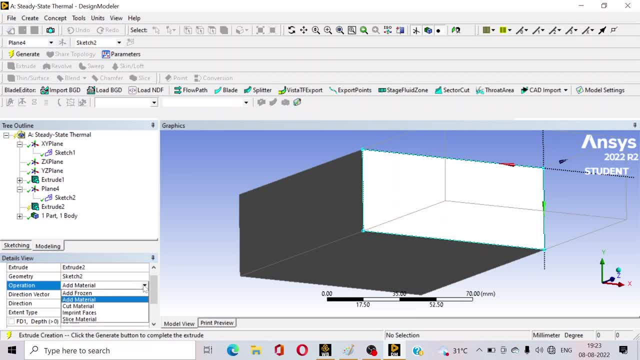 many kind of operation you can do with extras, extrusion, okay. so we will select add material. card material, slice material, add frozen. we will select add frozen. why, if you see, if we select add material, then nothing but it one single body will be created. but if we select add frozen, two different solid will be created. in our case. these are the two. 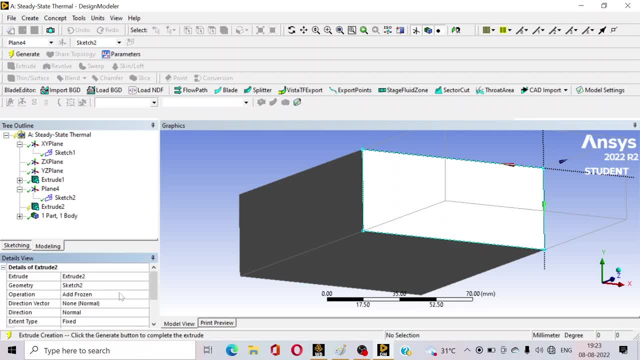 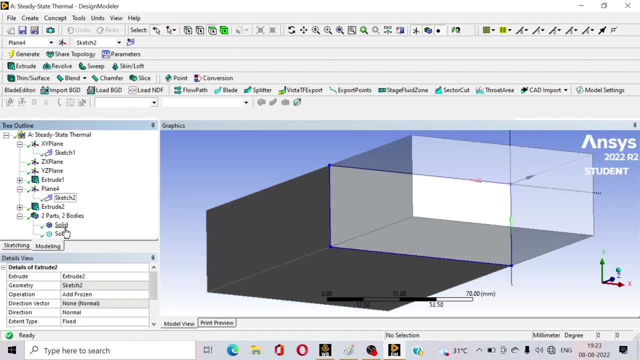 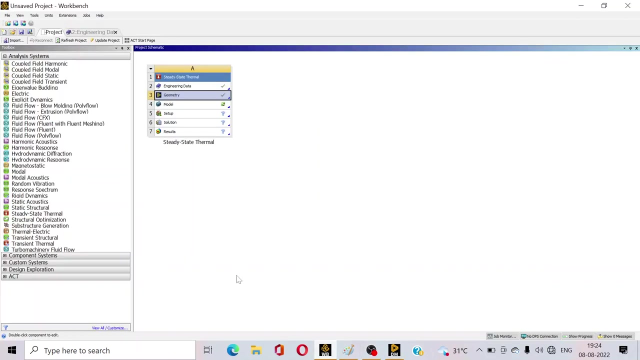 different solid, so we'll click add frozen. okay, now click on generate. okay, you can see that here two body are generated. one is this one, another one is this one. okay, so from drawing part we have done okay, now just go to the main slab. okay, double click on model for the next part. 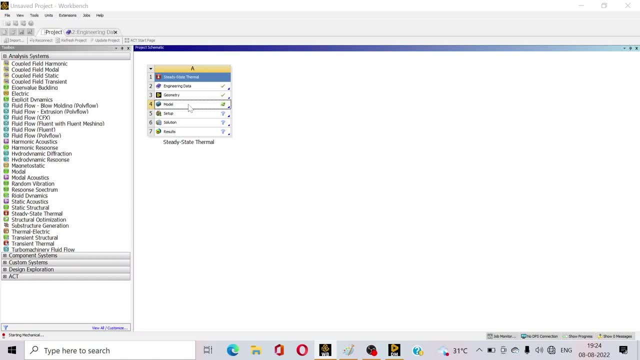 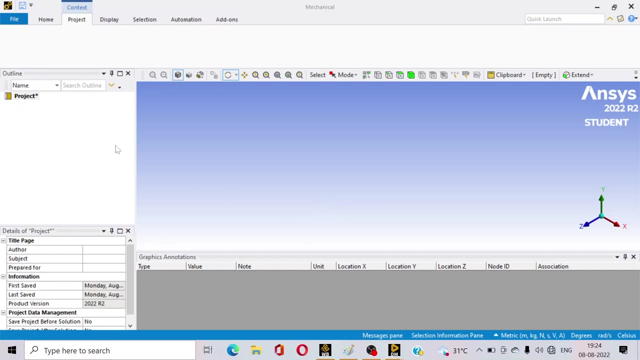 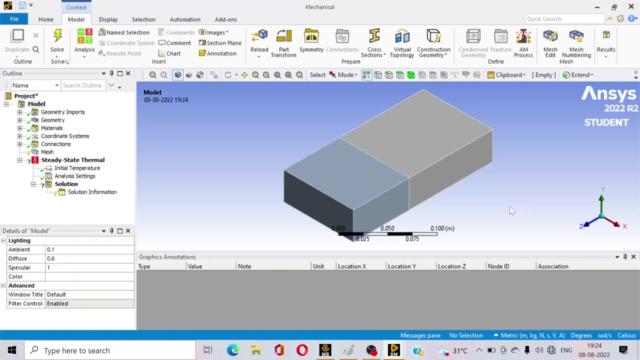 it will take a time. please wait. here it is. you can see. you can see, here is the main object and this is the copper slab and this is the bakelite slab. right and heat will be conducted from this direction. do this direction, this to this right. so just see the problem once again. 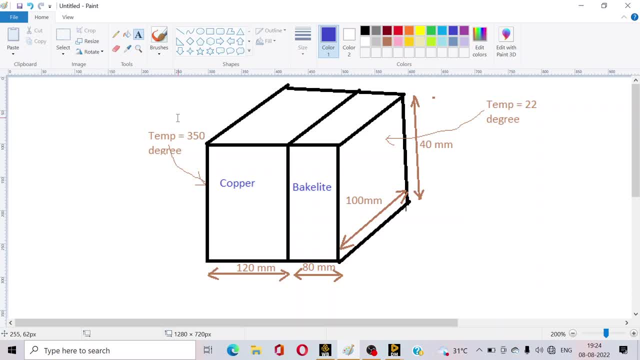 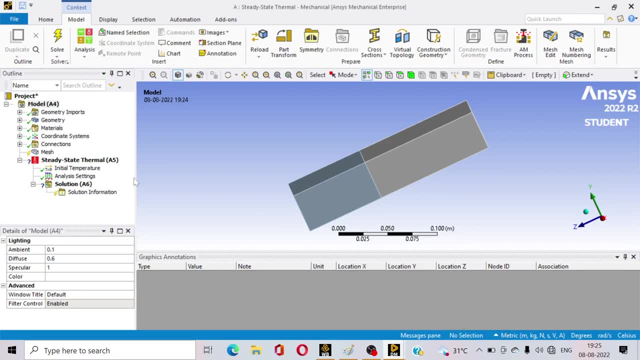 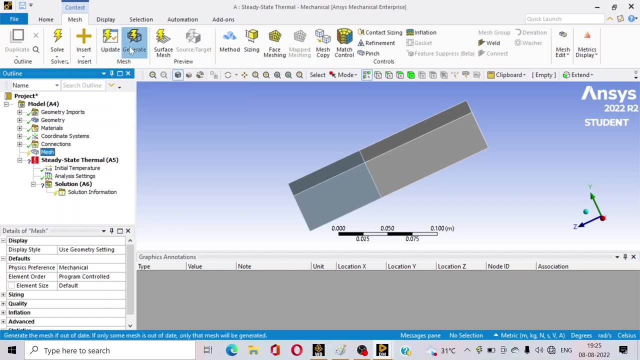 and the copper surface the temperature is 350 degree and at the bakelite surface the temperature is 22 degree. okay, now go to the problem. first of all, we have to create the maze. so go, click on the maze and just click generate. automatically mesh will be generated, you can see. now go to the steady state: thermal. 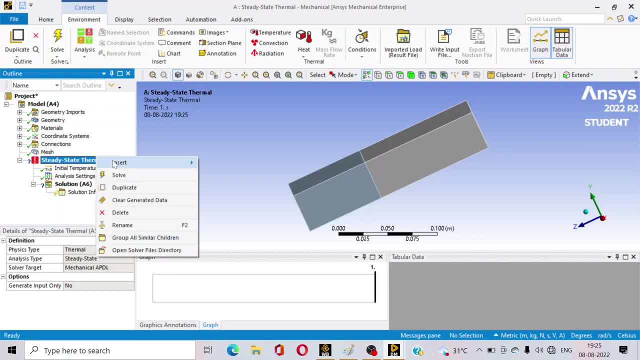 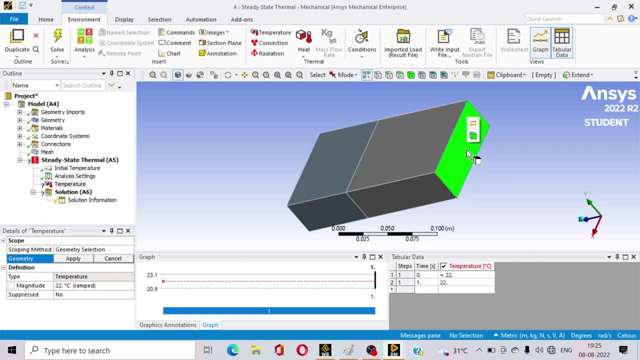 just click on it and right click, go to the insert, go to the temperature and just select this surface. just select this surface, this is the copper surface, right and apply. and the temperature: just change the temperature here. just type 350, okay, and enter so 350 degree centigrade temperature we have assigned for this. 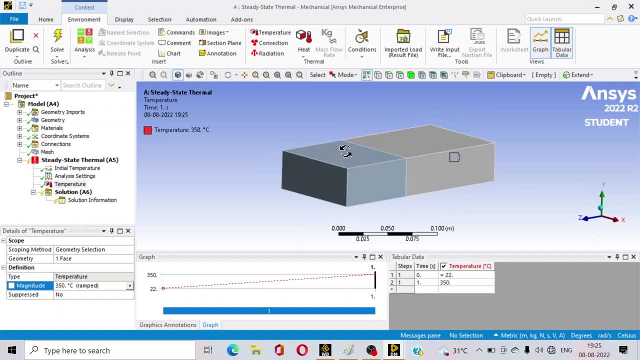 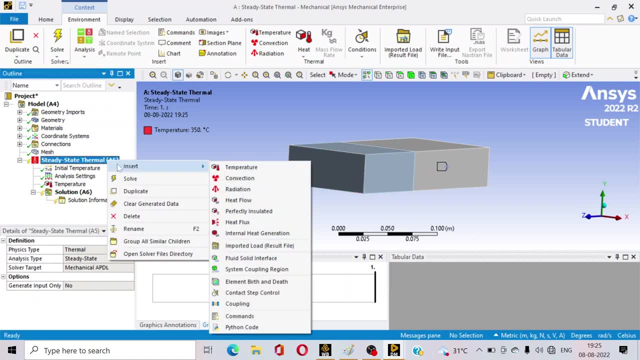 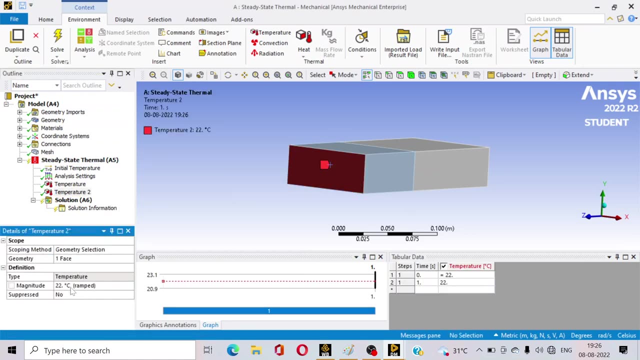 surface of the copper slab right and then again this is the bakelite slab right. so again go to the steady state, thermal right click, insert temperature and just click on it and apply and the temperature. just change the temperature here. just type 350 this surface and apply at this surface. temperature is 22 degree. it is already selected. 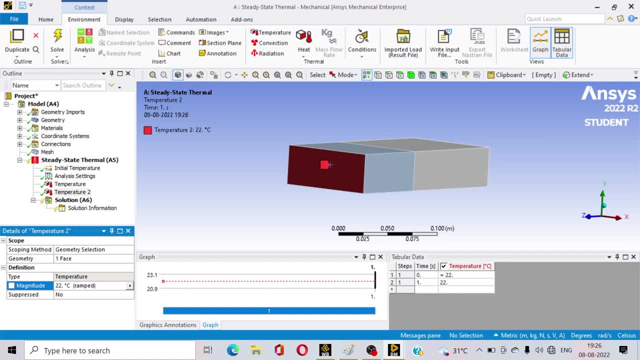 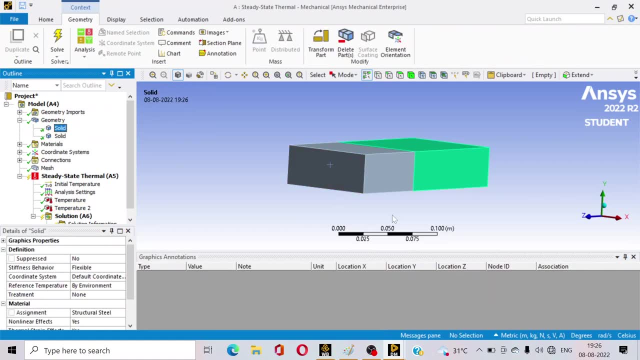 okay, this, we have done our part. now go to the geometry. we have created two solids. one is this one, another one is this one, but we have not assigned the material, so that we have to assign the material. you can see that this is the copper body, so just. 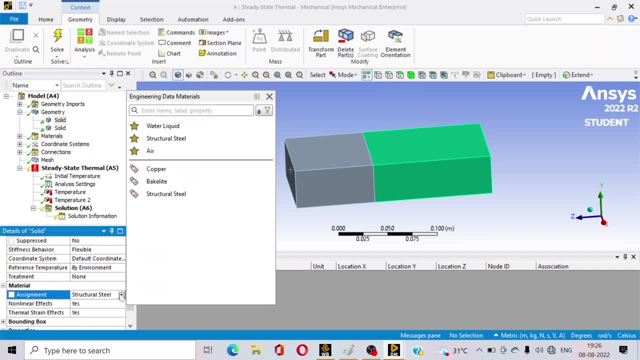 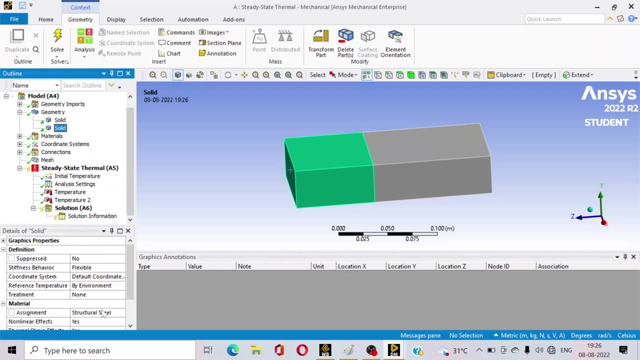 go to the assignment and just click these sections and you can see that at engineering data section we have selected copper and bakelite. so it is showing here. so just click on copper, because this solid is made up with the copper, and then go to the another solid and just go to. 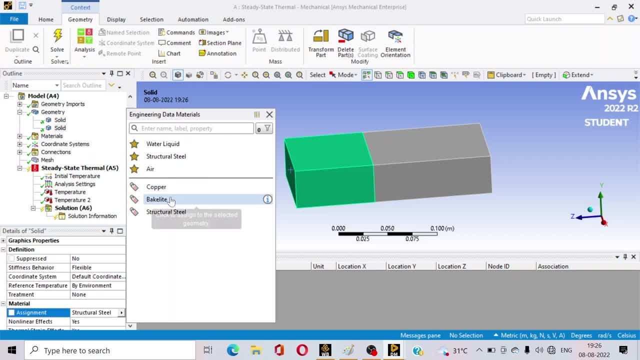 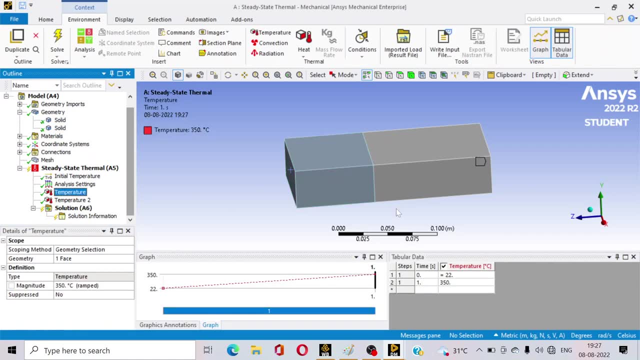 the assignment and just click on bakelite. okay, so we have assigned the material once again and we have assigned the temperature, and we have assigned the temperature and we have assigned the temperature and this surface is 350 degree. you can see here and this surface, the temperature is 22. 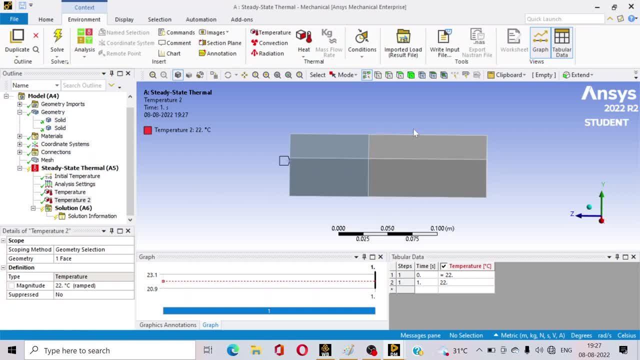 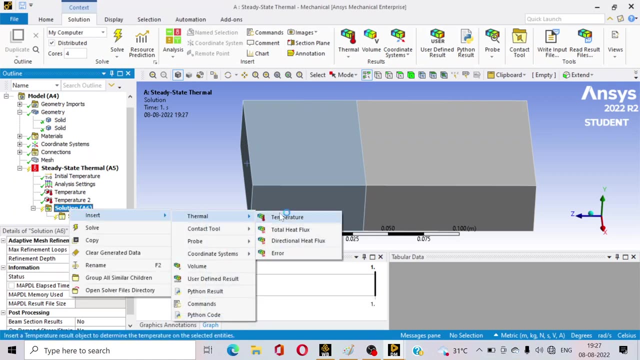 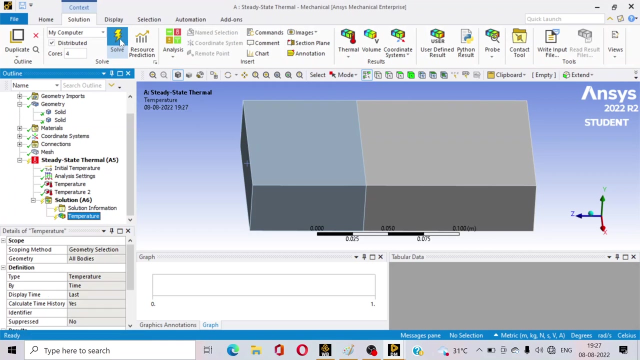 degree, that is, ambient temperature. okay, now we have to analyze this problem and we have to determine the temperature at the junction of these two block right, okay, now go click. click on the solutions. right click, insert thermal and temperature, because we want temperature right now. click on solve. 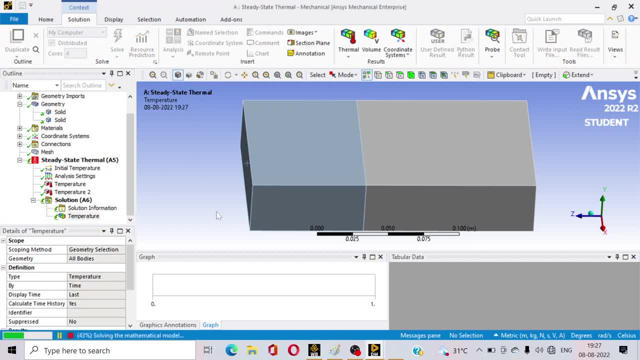 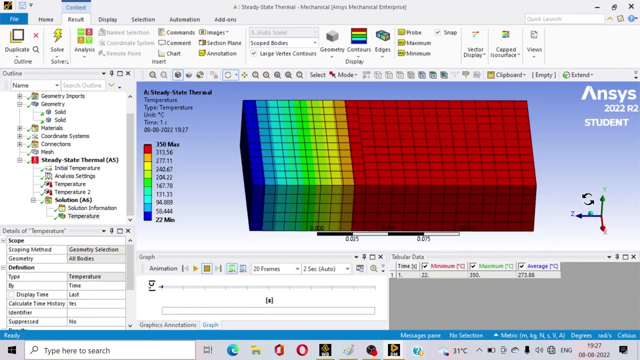 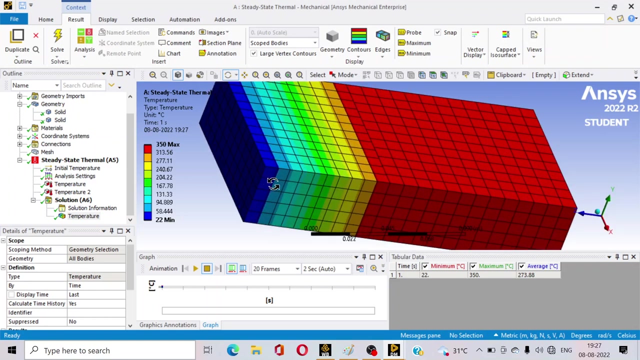 it will take some time. obviously, problem is solving. you can check the progress here. right again, the speed of the solving. solving problem is depend upon the configuration of your pc. and here it is. you can see, here it is. you can see different color for different temperature is already here and you can see the temperature graph here. 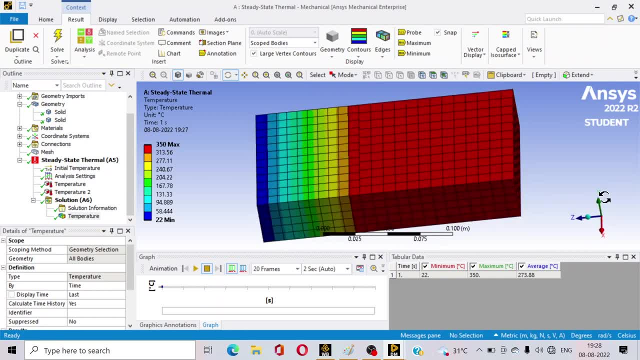 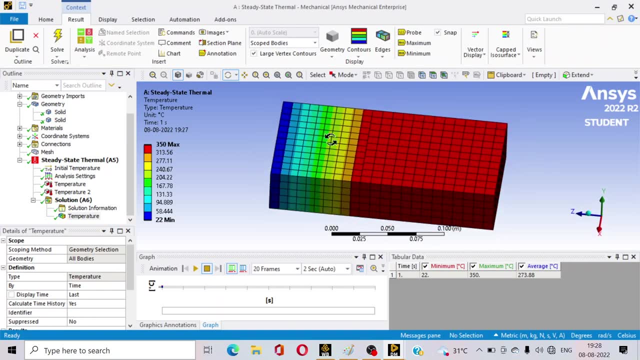 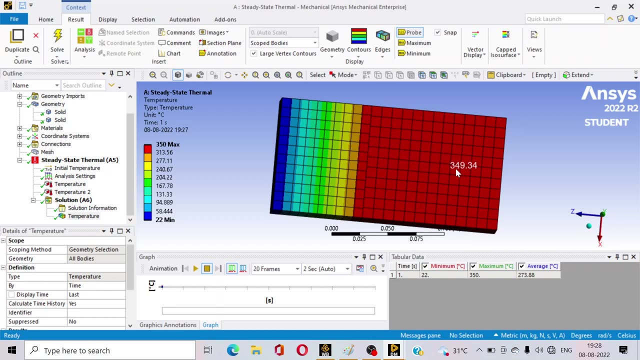 so at this surface the temperature was 350 degree. at this surface it is 22 degree. okay, now if if you want to check the temperature at any point of the body, then just click on the probe. okay, just move the cursor. you can check the temperature at different section it is showing. 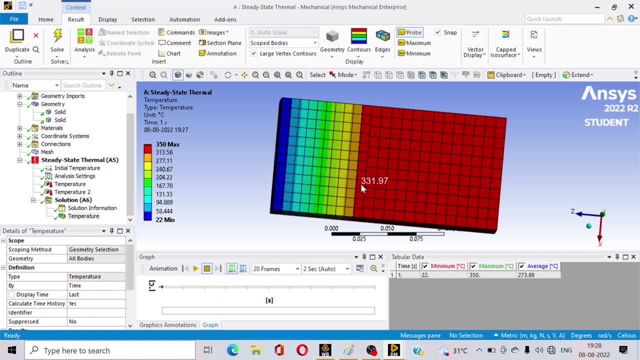 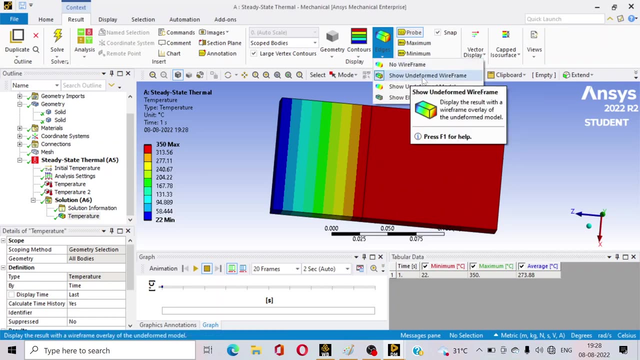 okay, right. so what is the temperature at the junction of these two block? now go to the edges and just click there. so now go to the sensor and then click on the problem. ok, and then go to the. just click this right. click this so undeformed wireframe right, so that you can see that at the 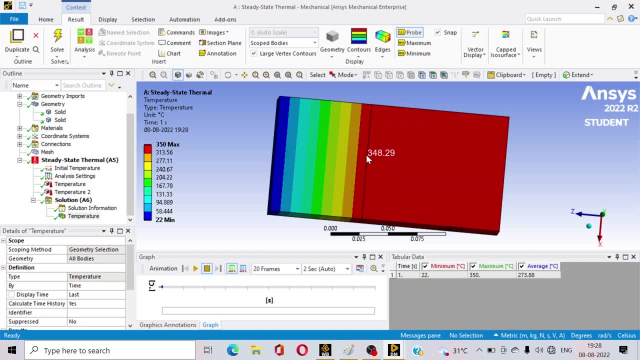 junction of two block. the temperature is 348.29 degree. okay, 348.29 degree, and you can also check the temperature at any surface you can check. check it here. the temperature is more and you can see that, as this is a copper and thermal conductivity of the copper is more. 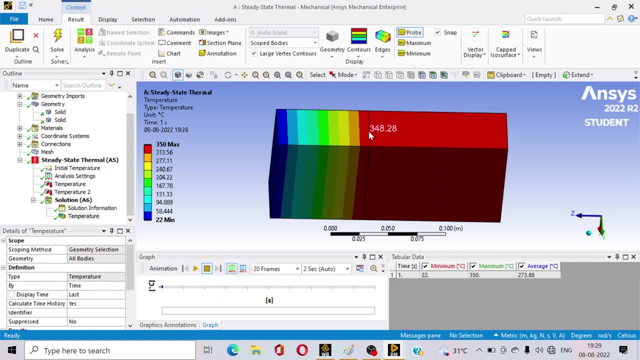 so that the heat transfer take place very rapidly, so that the temperature reduction is minimum here, but here the temperature reduction is more, because this is the kind of insulator, it is bakelite, and thermal conductivity of bakelite is lower side, so that here the temperature is decreasing very rapidly, and here it is 22 degree, what we have assigned, and you can.